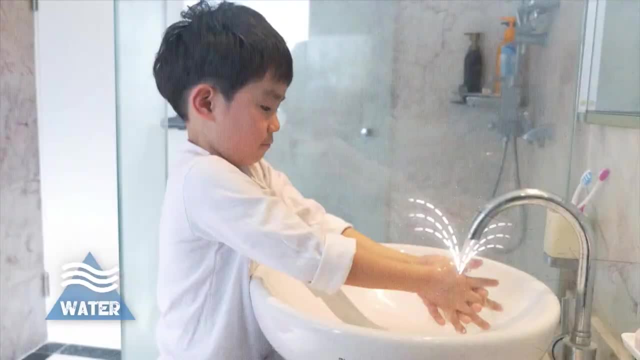 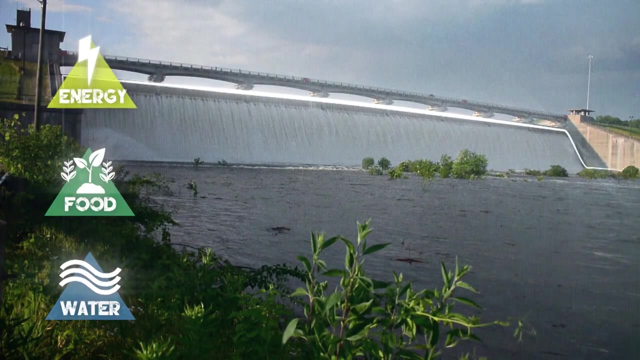 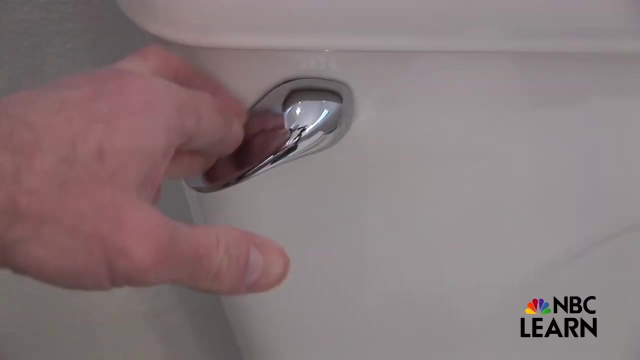 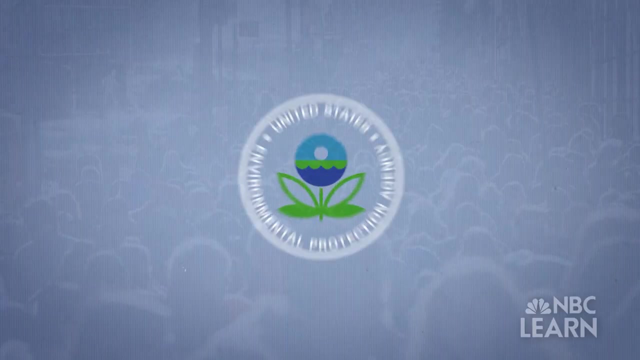 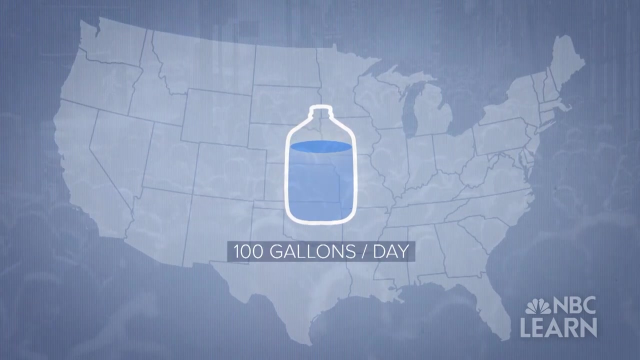 Wastewater: It's what gets flushed down the toilet, rinsed down the drain and produced by places such as factories, workplaces and homes. According to the US Environmental Protection Agency, the average person uses about 100 gallons of water a day, with almost. all of it turning into some form of wastewater. Of the 100 gallons per capita per day of wastewater we produce, we are drinking about a gallon per day per capita. Essentially, wastewater is the one gallon of human waste produced per capita per day, diluted with 99 gallons. 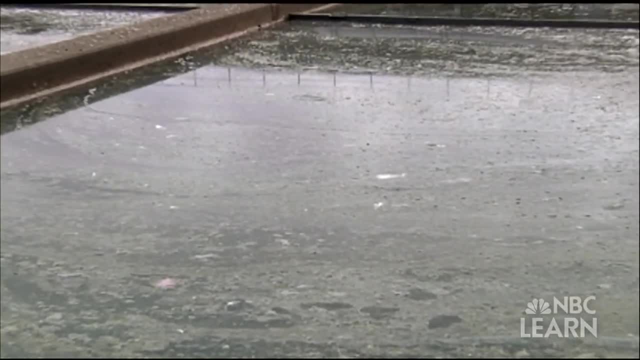 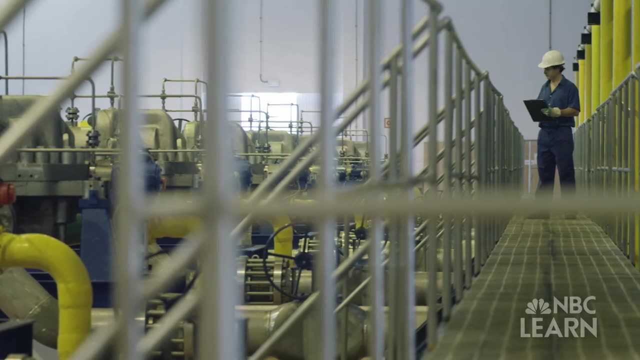 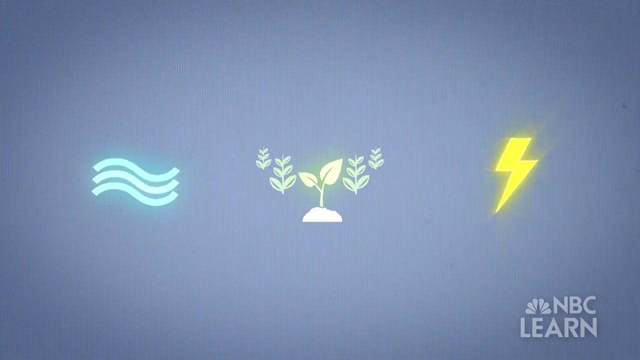 of non-human waste. Because wastewater contains pollutants and contaminants, most communities send it to treatment plants to be purified, The process: The water has to meet federal, state and local standards before it's released back into the environment. Wastewater is one part of the human water cycle. 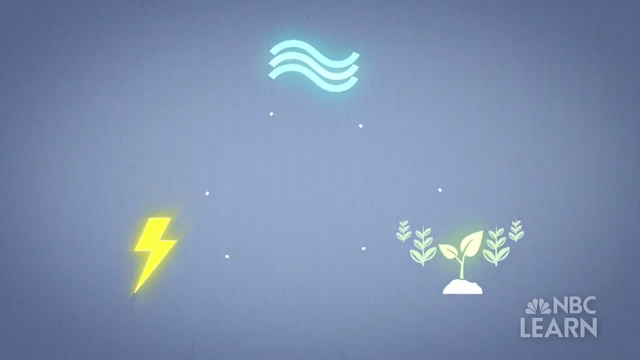 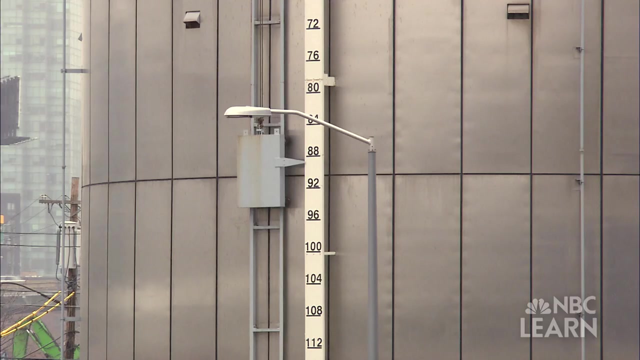 which describes the many ways people interact with nature's hydrologic cycle to meet our needs for water, food and energy. While water treatment plants are a necessary part of public health and environmental safety, they require a great deal of energy and resources to operate. 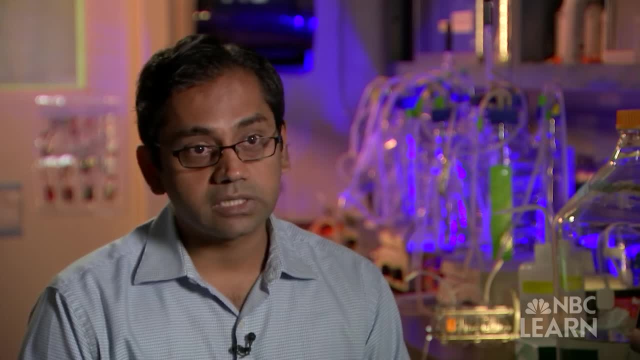 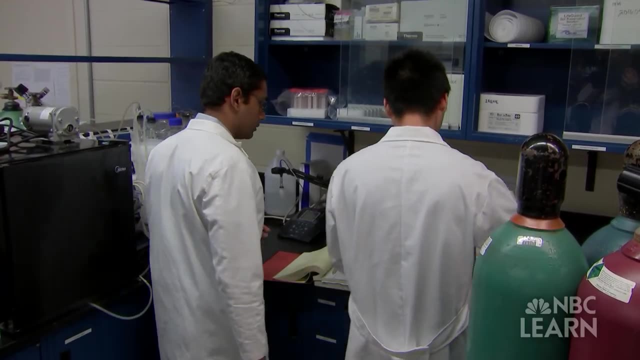 In the US, we devote about three to six percent of the national energy budget on the enterprise of clean water. Kartik Chandran is a professor of earth and environmental engineering at Columbia University and funded by the National Science Foundation. He investigates new, more efficient ways to 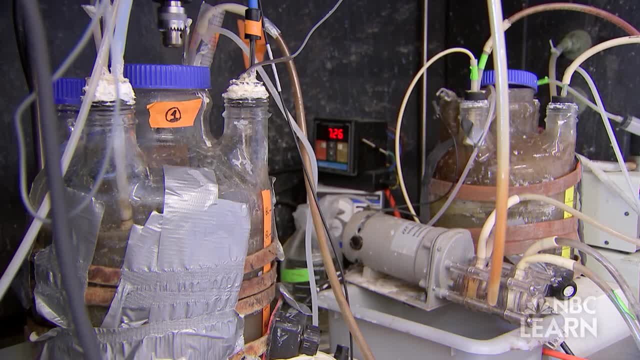 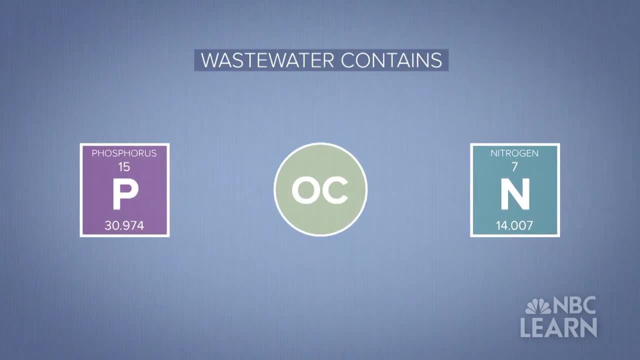 treat wastewater. Wastewater contains elements such as phosphorous, organic carbon and nitrogen, which are often removed during the treatment process. Let's start with nitrogen. When we want to remove nitrogen, we want to remove it in a different way. When we remove nitrogen from wastewater in addition to the organic carbon. the energy footprint of a wastewater treatment plant essentially doubles At the Newtown Wastewater Treatment Plant in Brooklyn, New York. treating wastewater involves several steps. First, the system separates floating matter and solids from the water. The remaining sewage then enters an aeration tank. 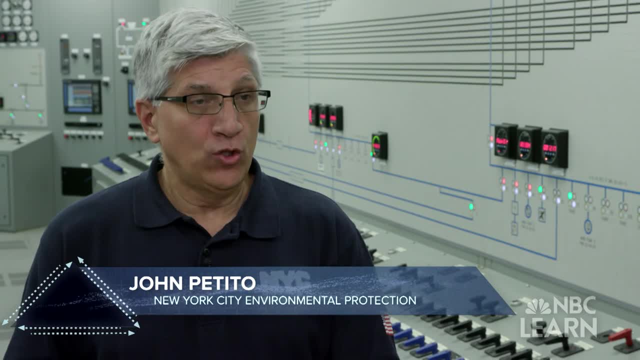 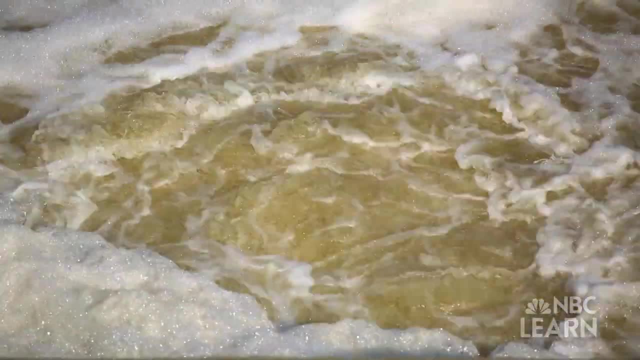 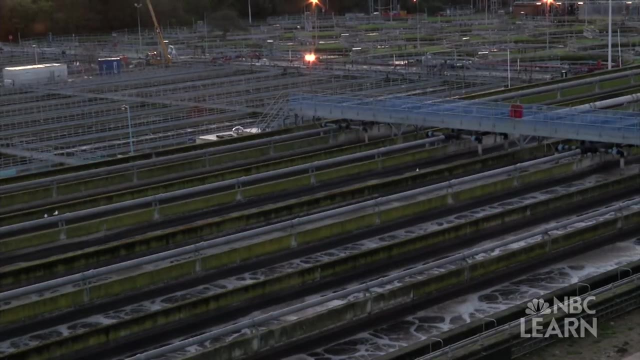 What we do in aeration tanks is we supply oxygen to microorganisms that actually treat the sewage. Local microbes for wastewater treatment require oxygen to degrade organic pollutants. The resulting sludge is further treated and, in its final step, the water is disinfected. 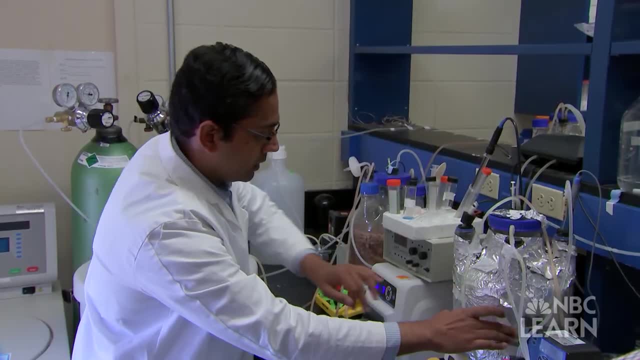 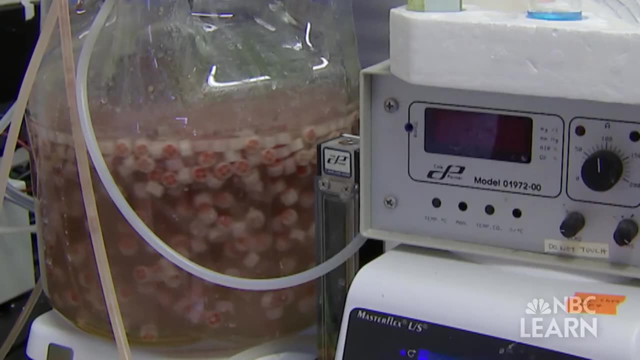 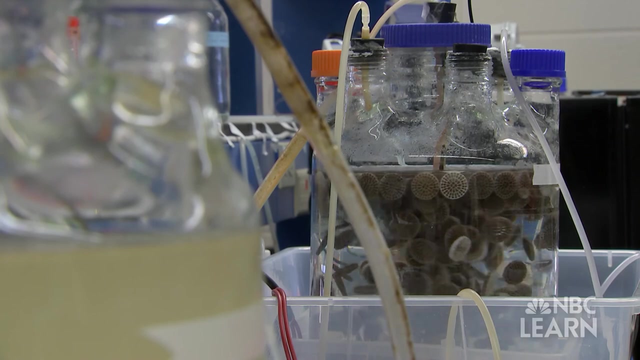 Chandran is trying to reduce the amount of energy used. in this process, He uses a type of bacteria found in wastewater called anammox. These organisms don't need oxygen to remove nitrogen from wastewater, While traditional wastewater treatment often releases greenhouse gases such as nitrous oxide and carbon dioxide, using anammox bacteria 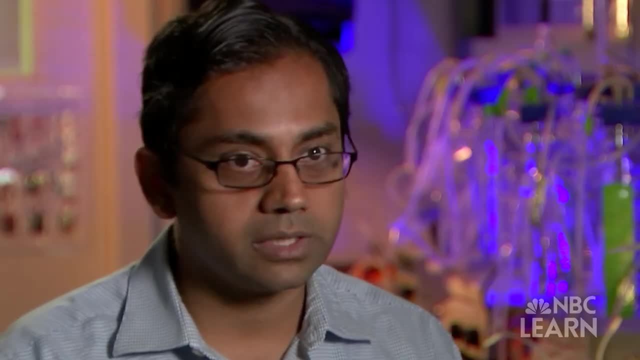 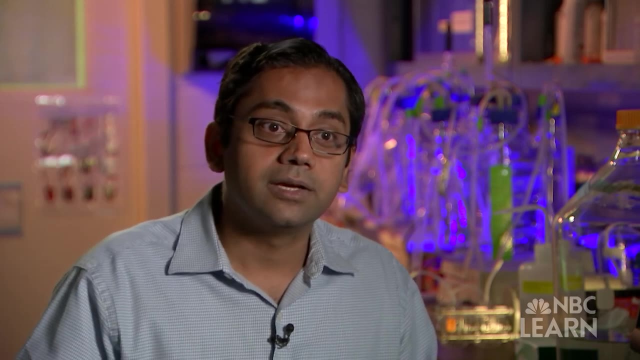 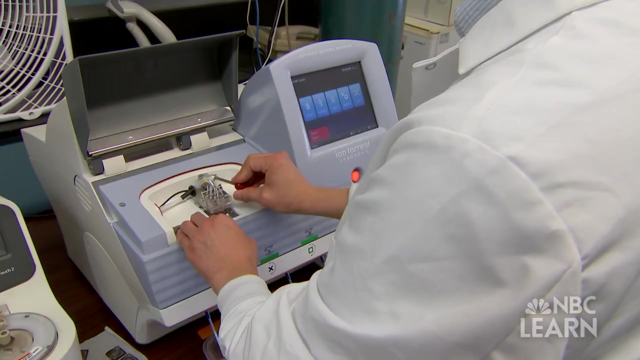 does not. They allow us to remove nitrogen at far lower energy costs and chemical costs. Not just that: we would save 60% in terms of aeration costs if we use the anammox model for removing nitrogen. Chandran and his team are also looking at ways to use wastewater's abundant chemicals. 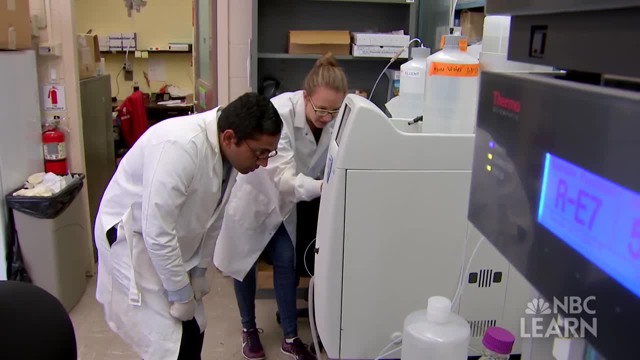 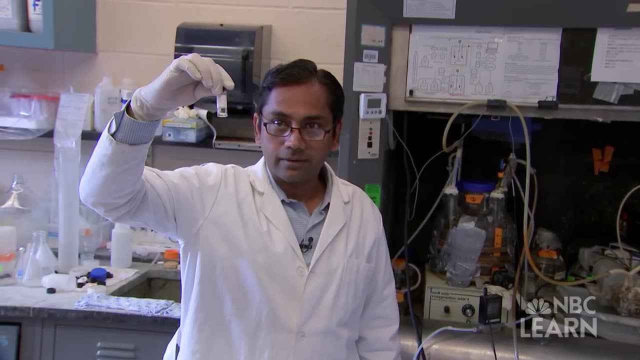 nutrients and other resources to produce energy. We have been able to convert this waste into energy. We have been able to convert the organic carbon in food waste, in sewage sludge, in fecal sludge, to biodiesel, which is a liquid fuel easily transported and easily used, directly used in diesel engines. 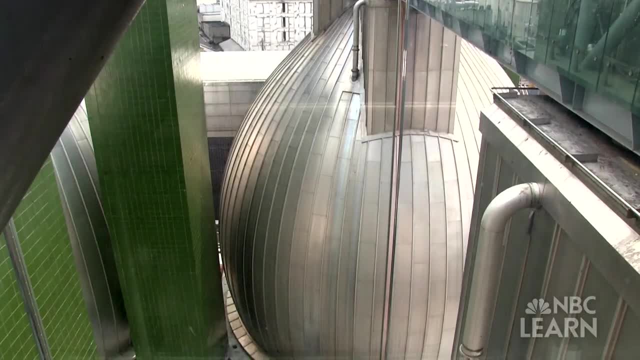 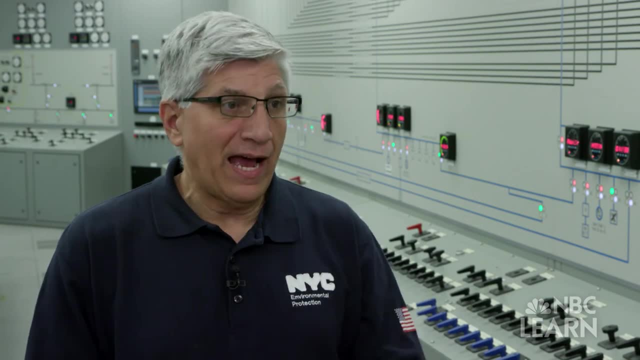 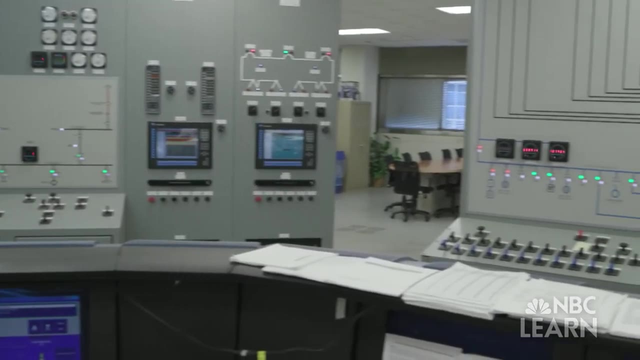 The Newtown wastewater treatment plant is already producing energy from organic material. The digesters are heated to about 95 degrees Fahrenheit. They act like the human body: They break down the organic material and we provide no oxygen And one of the byproducts- 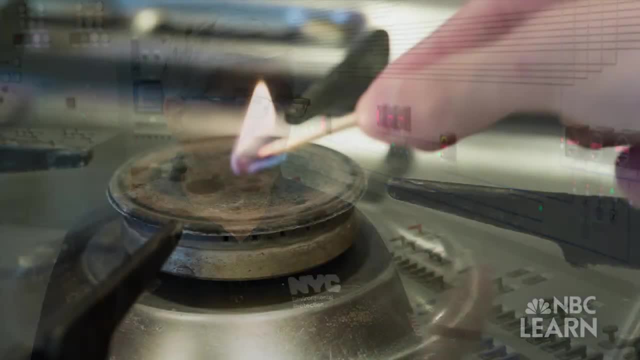 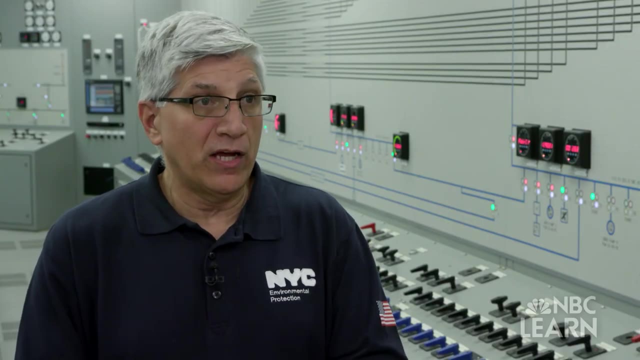 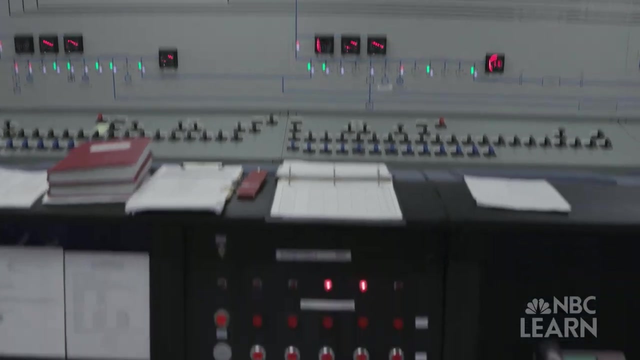 of the digestion process is methane gas. Methane gas is a common energy source. We are right now using a good portion of our digester gas to heat our boilers in our locations. The boilers are used for heating the environmental areas, the personnel areas, and they're also 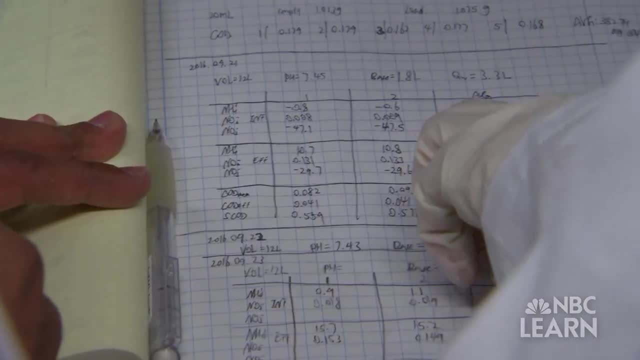 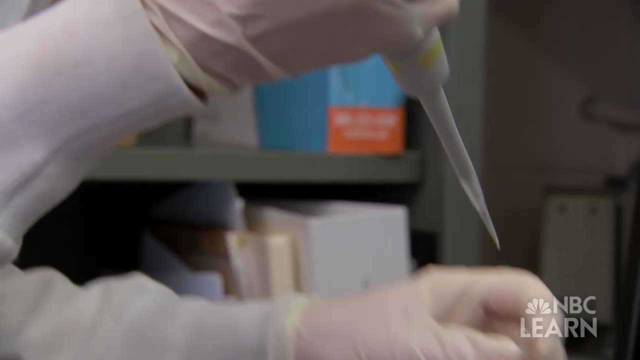 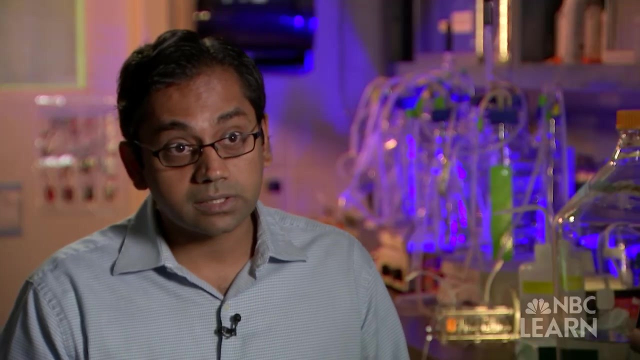 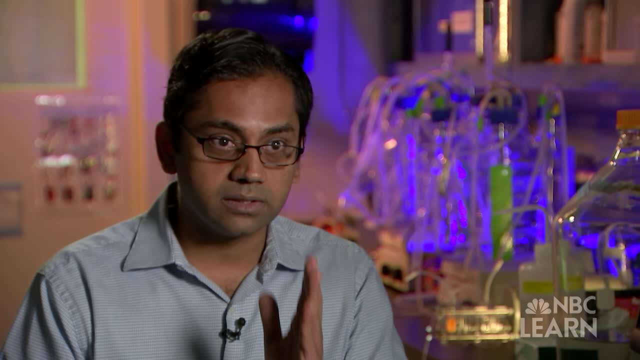 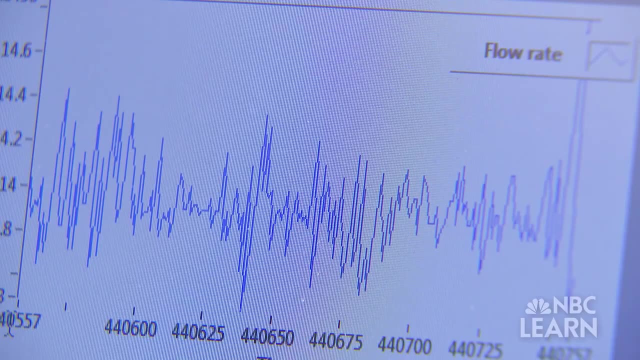 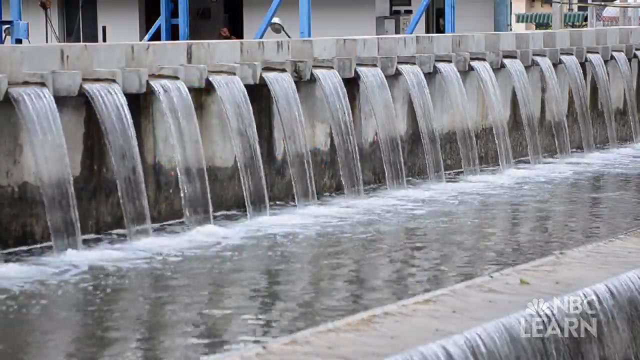 we are now able to address these challenges Not just one by one, individually, in isolation, but together in conjunction. that's a very sustainable model, As Chandran and his team help make the human water cycle more energy-efficient. they are also helping us see wastewater not as waste, but as a precious resource. you.